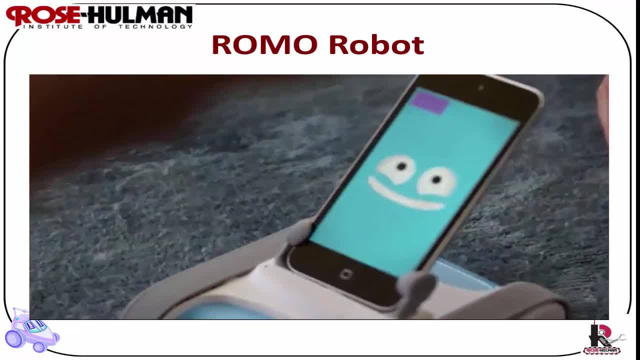 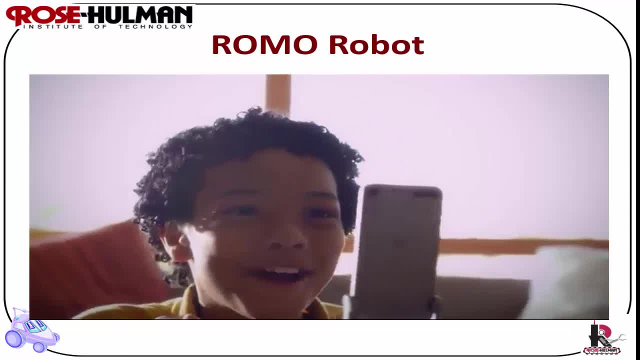 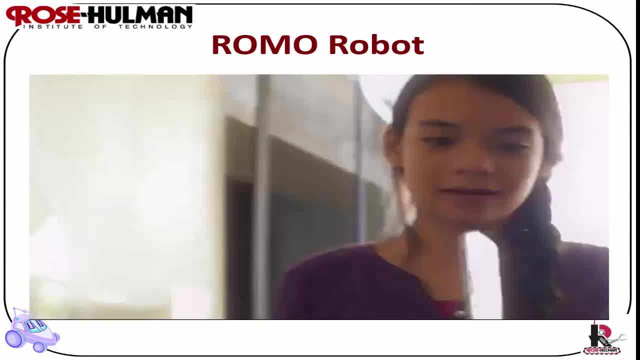 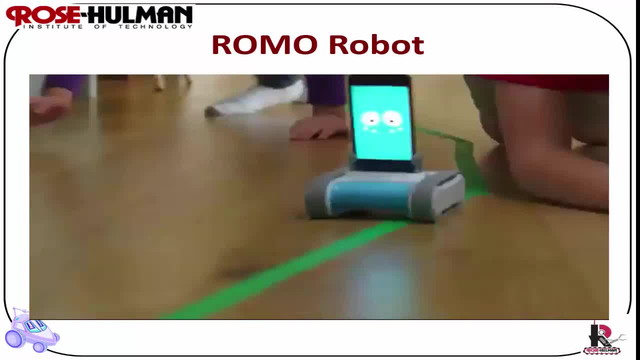 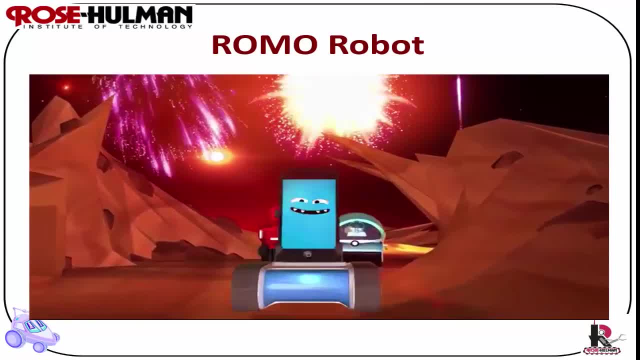 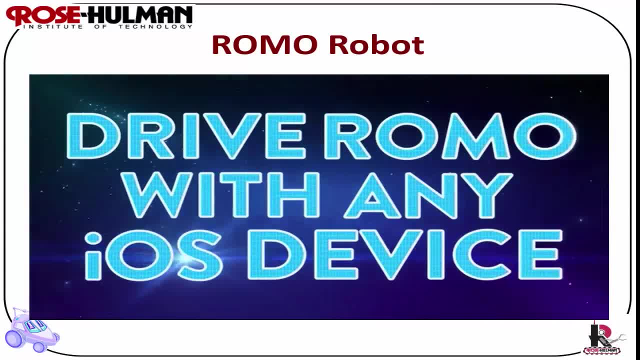 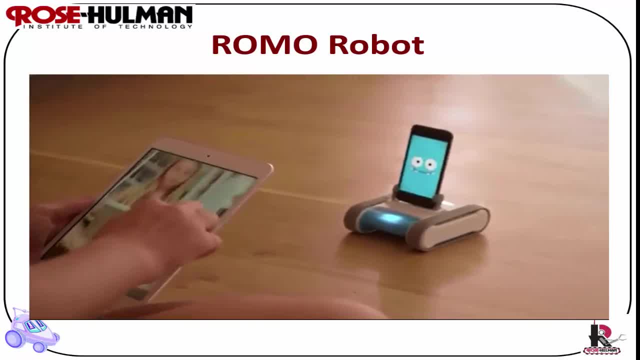 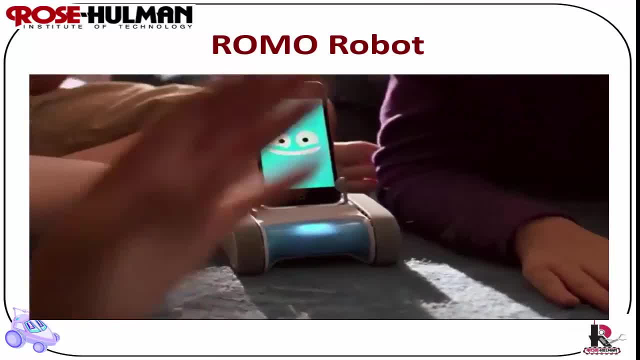 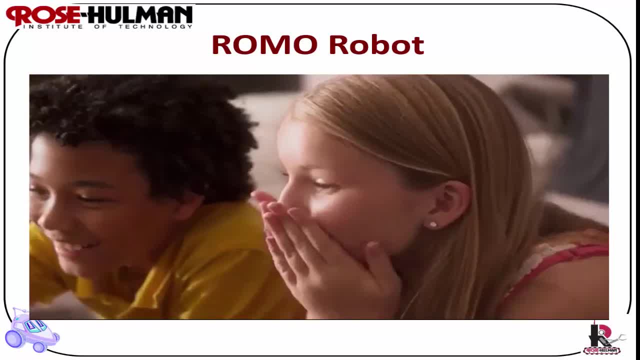 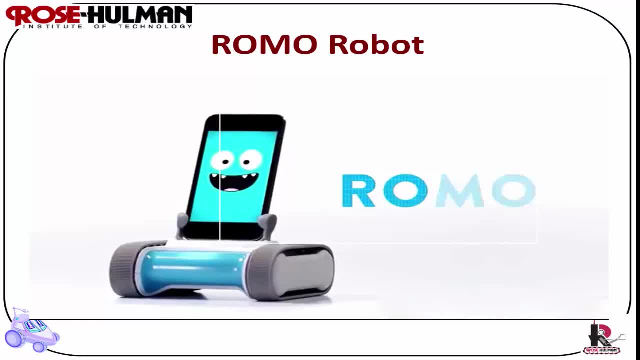 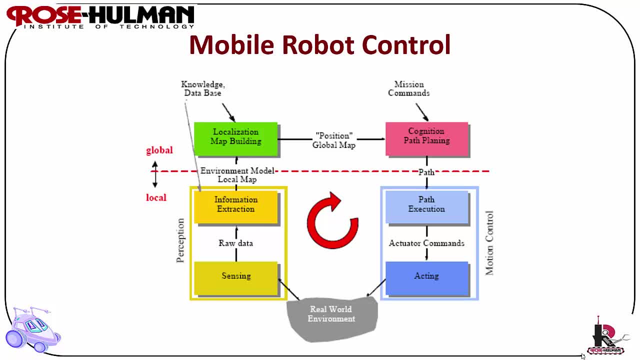 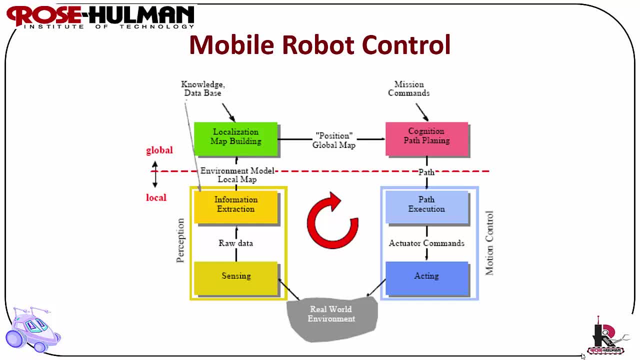 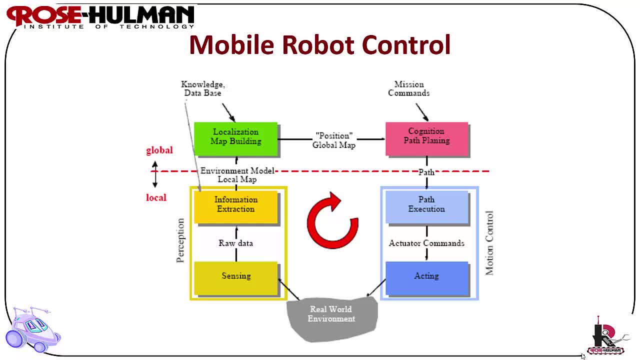 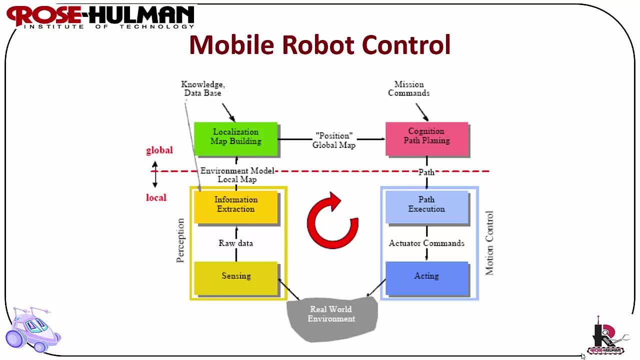 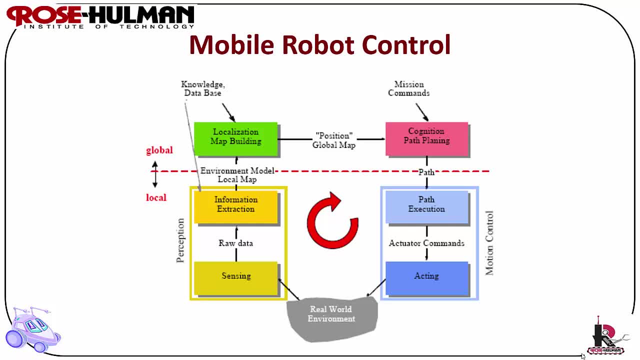 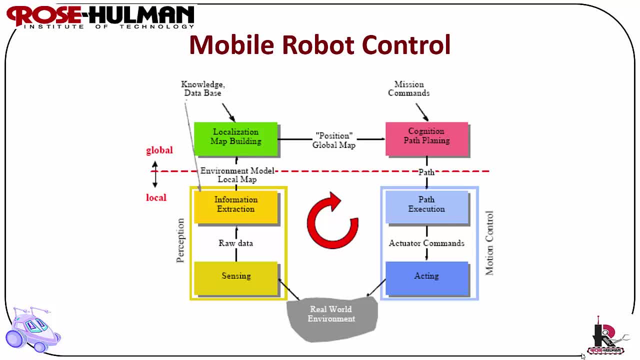 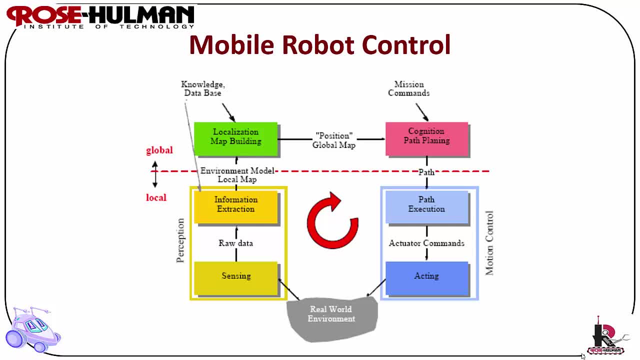 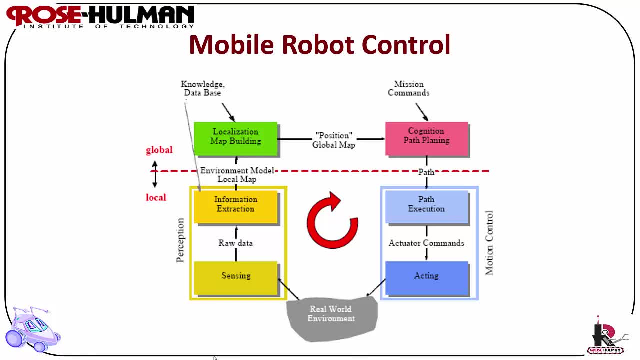 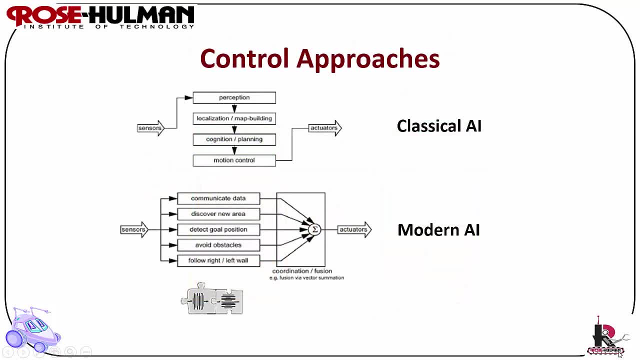 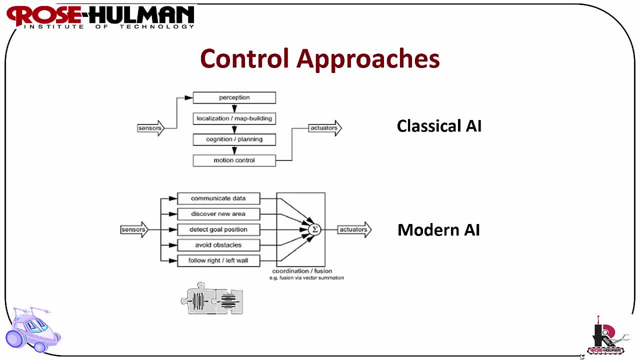 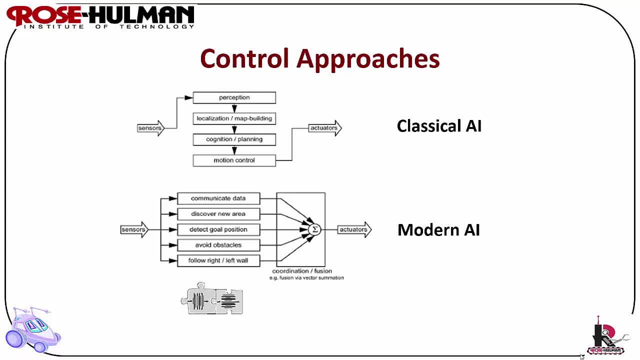 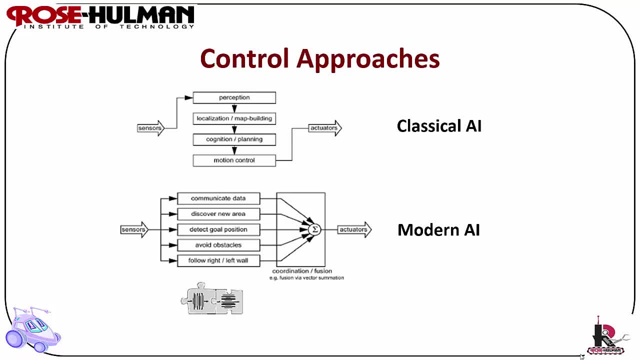 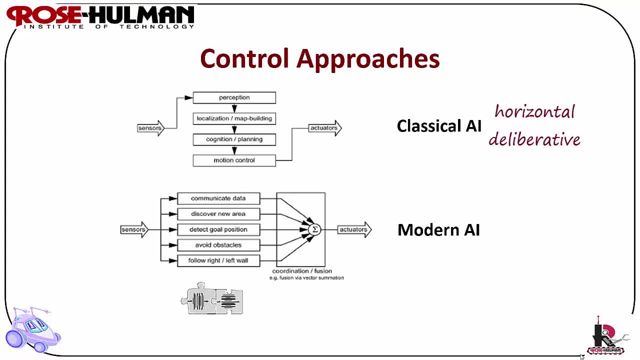 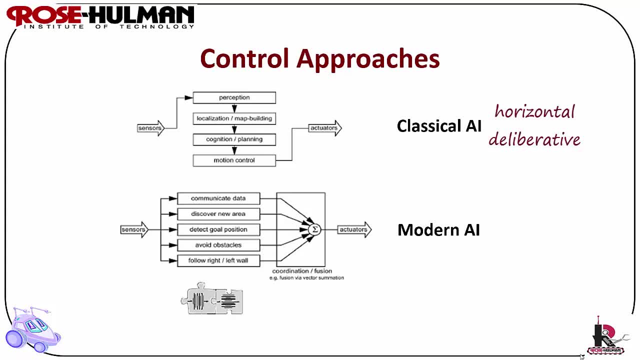 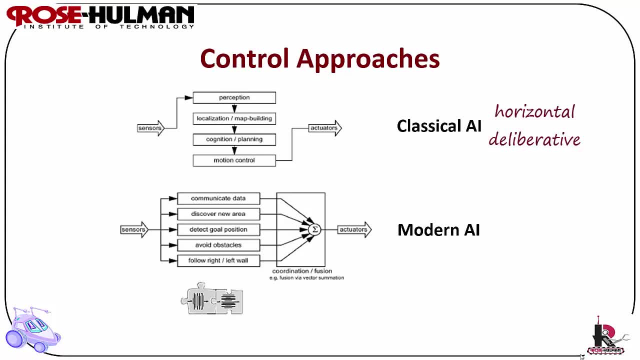 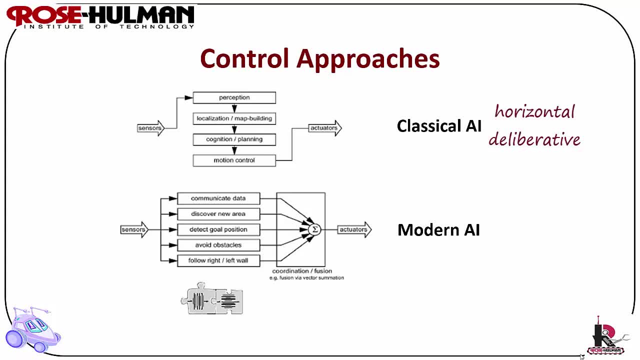 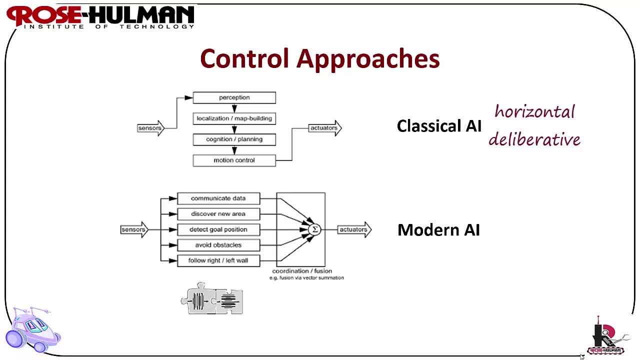 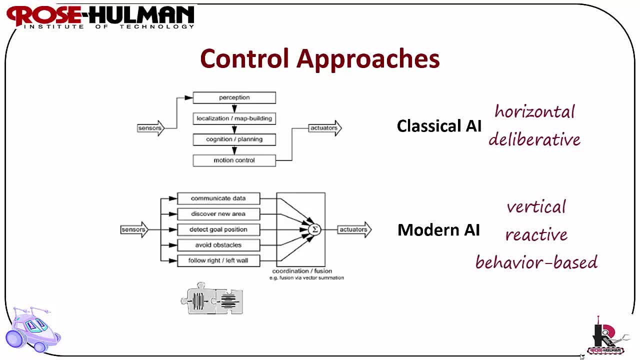 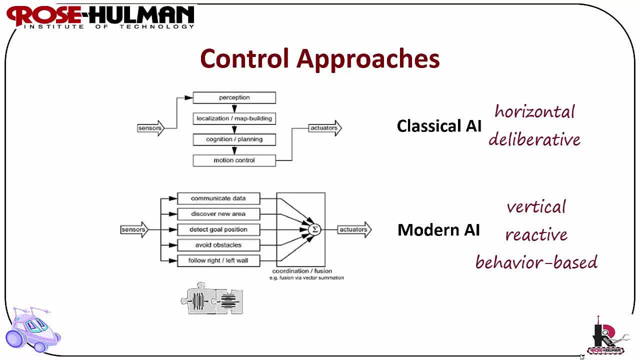 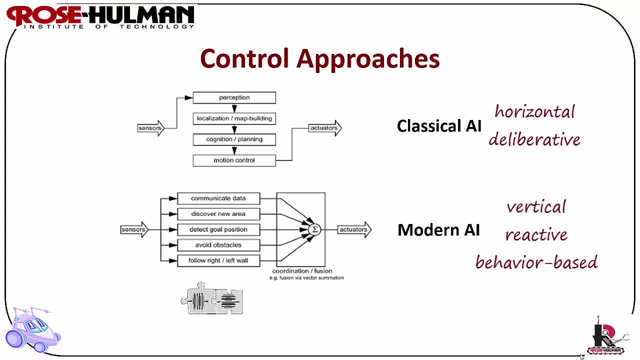 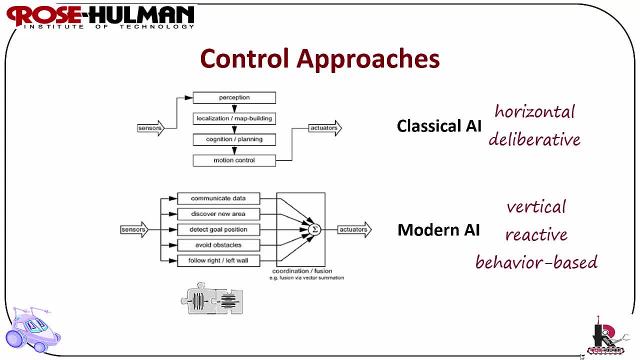 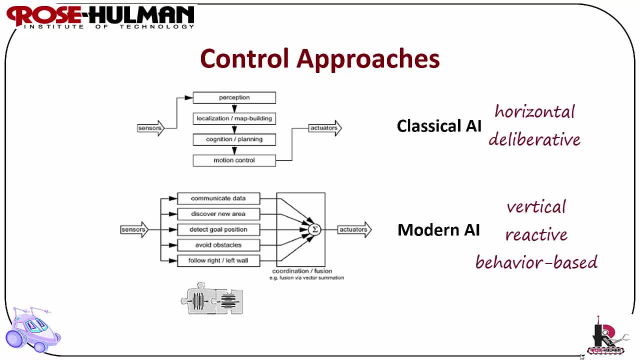 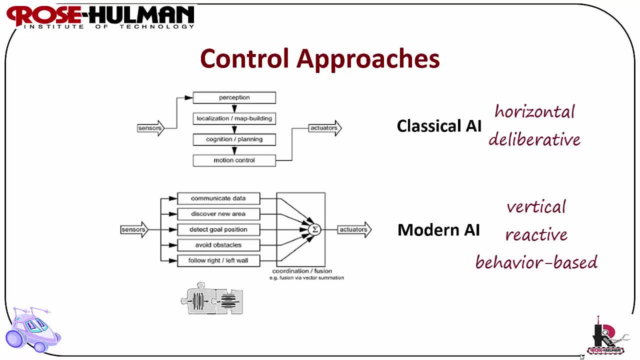 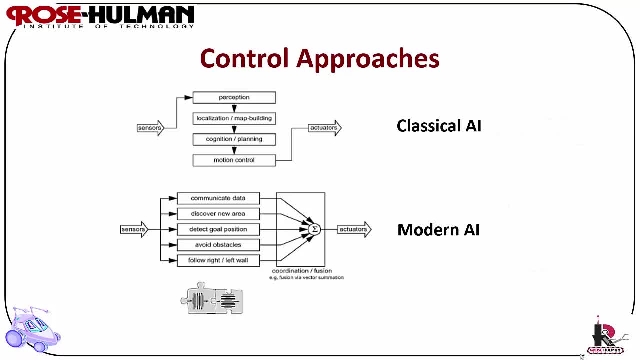 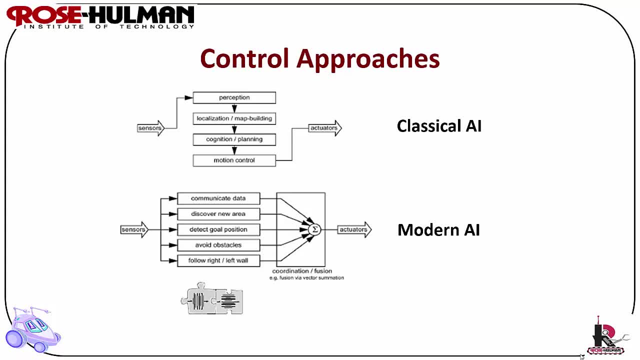 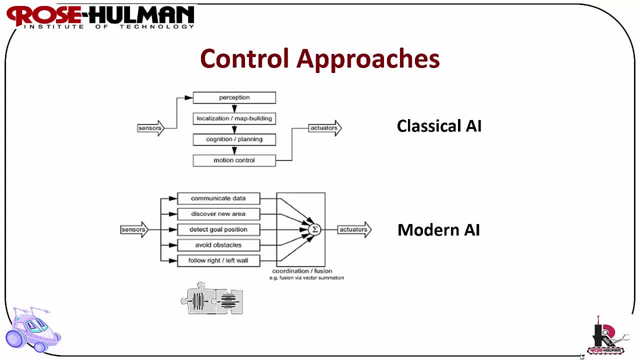 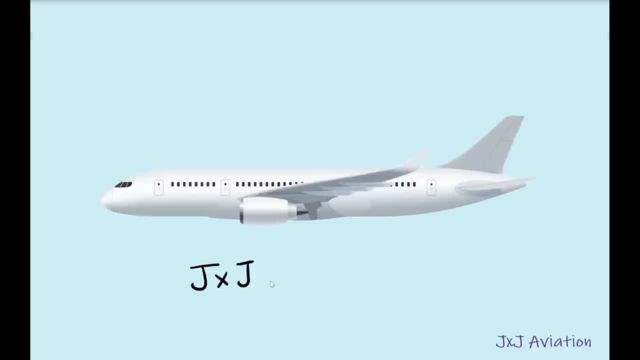 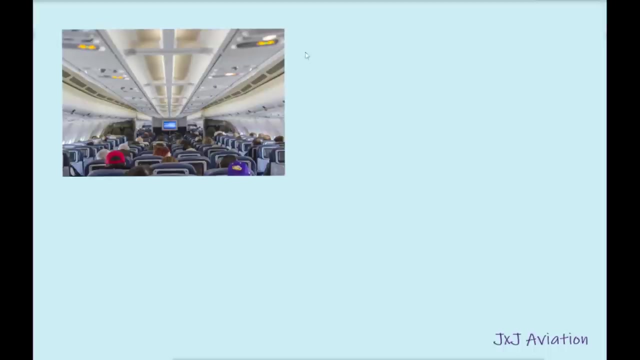 Hello and welcome to GXJ Aviation. In this video we will be looking at how the air conditioning system functions in an aircraft and what is an air cycle machine. First let's see why is an air conditioning system required in an aircraft. The air conditioning system provides cool air constantly inside the cabin and in the cockpit. 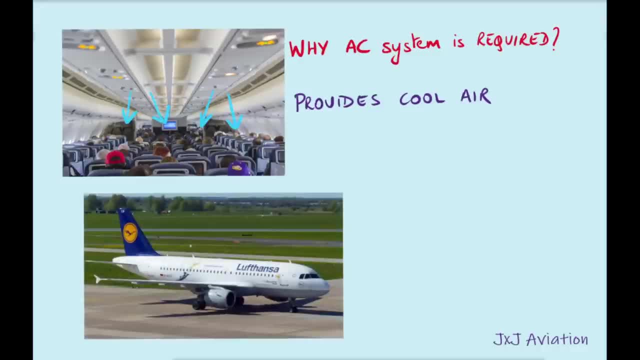 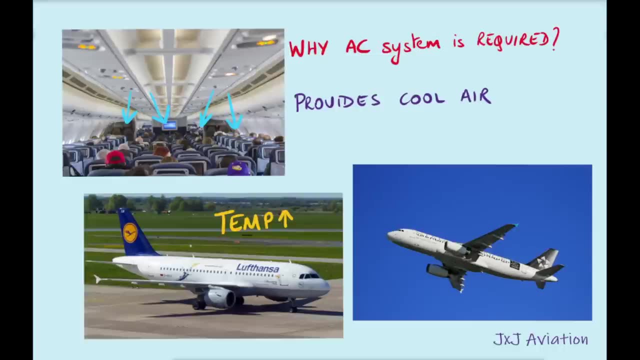 This is essential when the aircraft is on ground and the outside air temperature is very high, or if the aircraft is in flight where the outside air temperatures are very low. The air conditioning system improves passenger comfort and assists in maintaining the cabin pressure. How does the air conditioning system work?